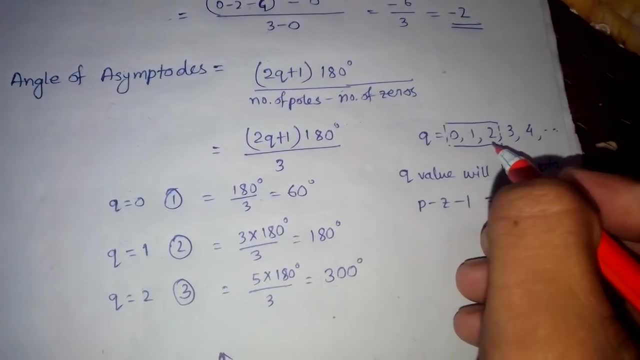 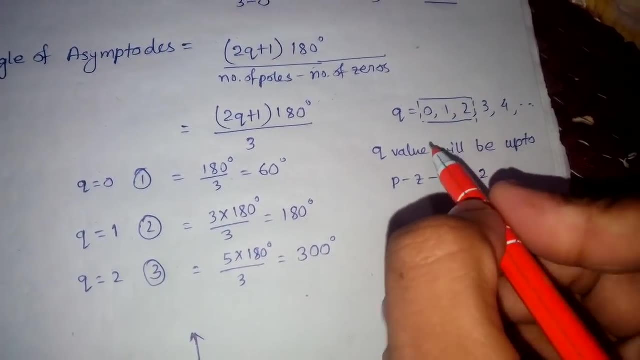 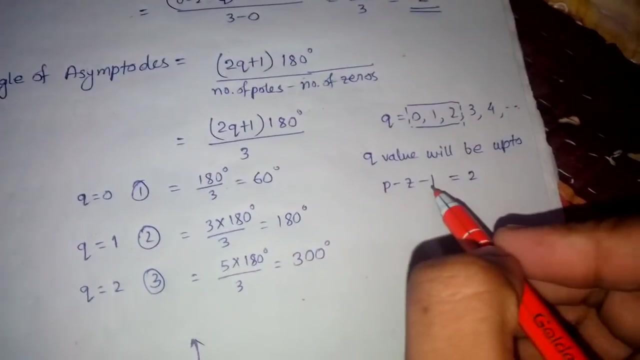 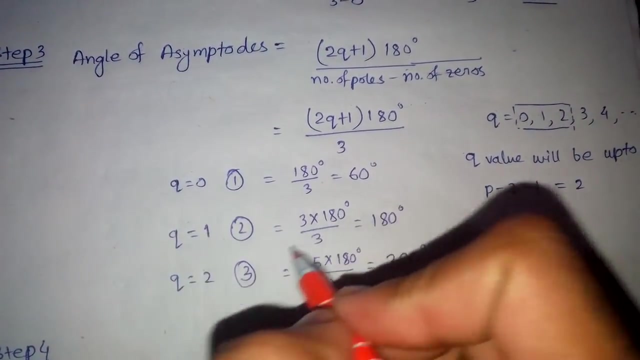 and after that you can find out that what is q? q value can go from 0 to any number, so q value will be up to. so how much we will take the q value? the q value will be p minus z minus 1. so here p minus 8 means 3, and 3 minus 1 means 2. so the q value will be 0, 1 and 2. so for this, 0, 1 and 2. 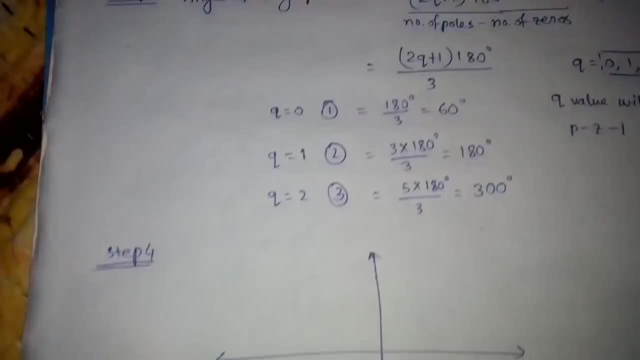 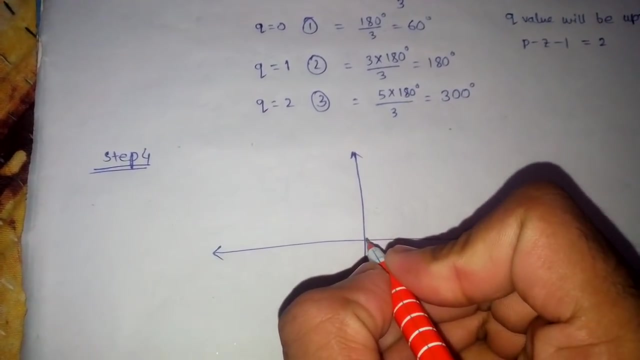 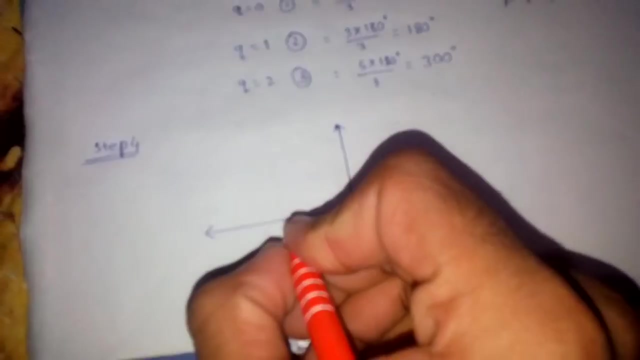 we have find out the angle of asymptotes here. after that we will go through the step 4. on step 4, what will we do? we will just point out the poles so we can see here that it is equals to 0. there there is a pole on. it is less than 0 and there is a pole on. maybe there is one, there is two. 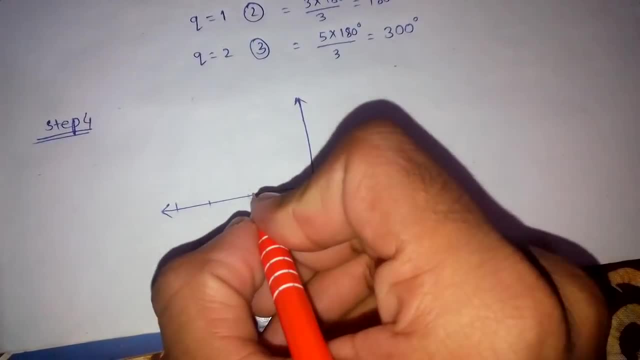 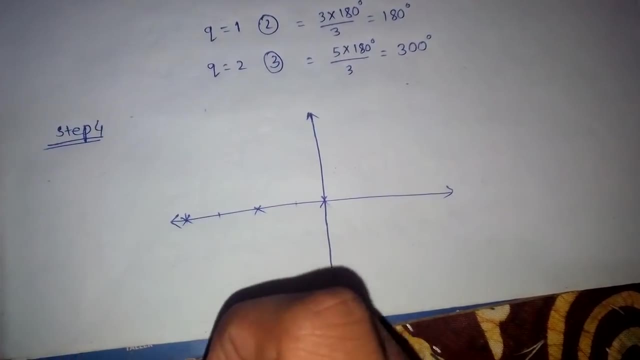 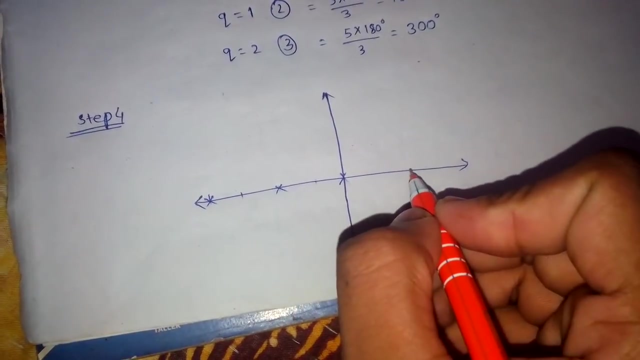 there is three and there is four, so here is a pole at minus two and here is a pole at minus four. okay, so we have to find out the root locus here, so from here we can see on the rh side of s plane. there is no poles or zero, so there will be no root locus. so we have to move on the next pole. 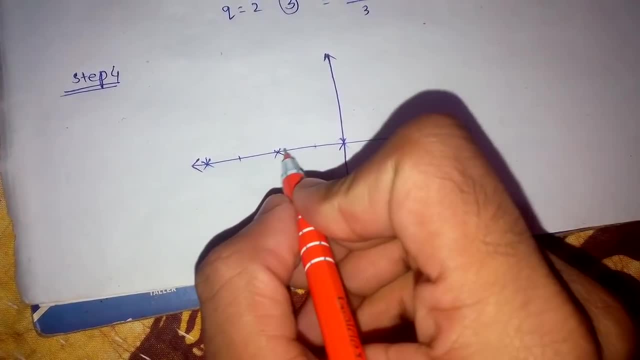 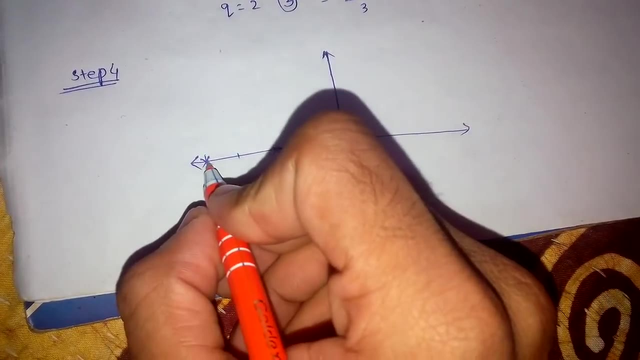 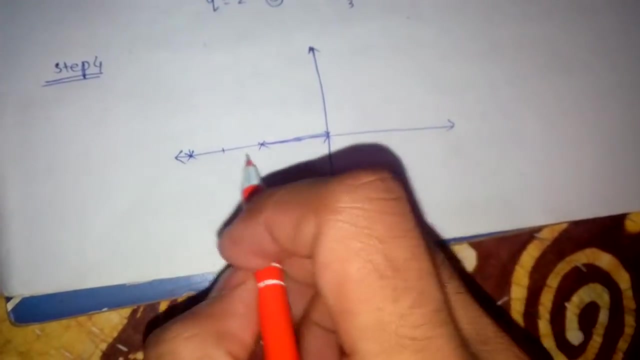 from the next pole you can see there is only one pole. so that is a odd number of poles. so there will be a root locus in between this and after that we will consider this pole. from this pole we can see there is two number of poles there. so this is the even number of poles. pole pair: okay, so we cannot. 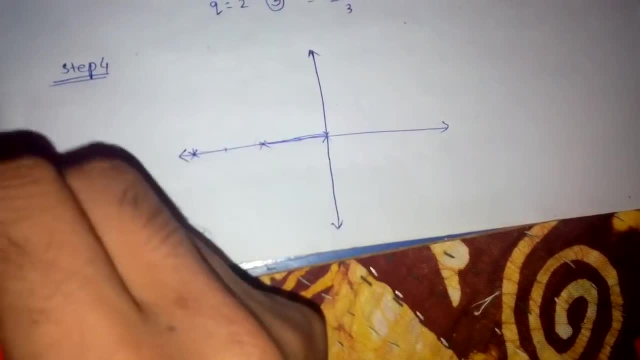 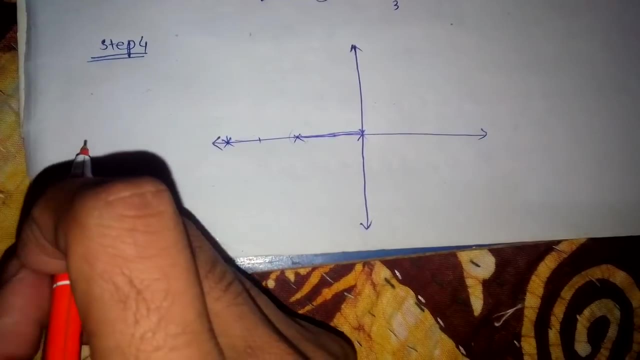 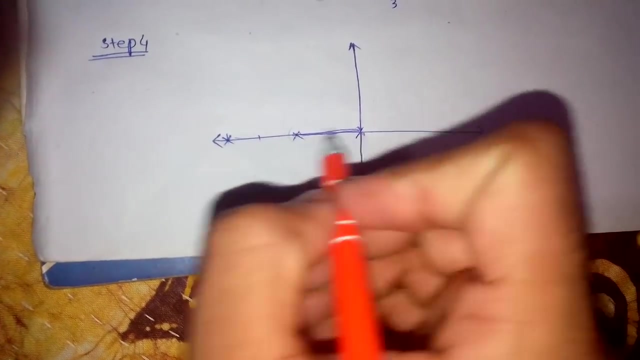 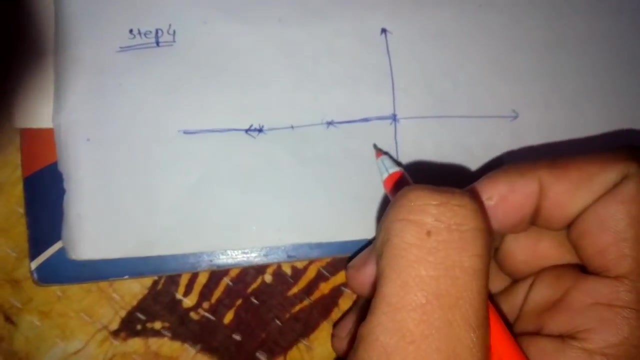 draw a root legus between this. so we will go for the next poles or zeros. so we consider that there is a zero or something. pole here. okay. on the infinity, from the infinite point, if we look after, is three poles okay. so from infinite to this there must be a root locus. so here is two. 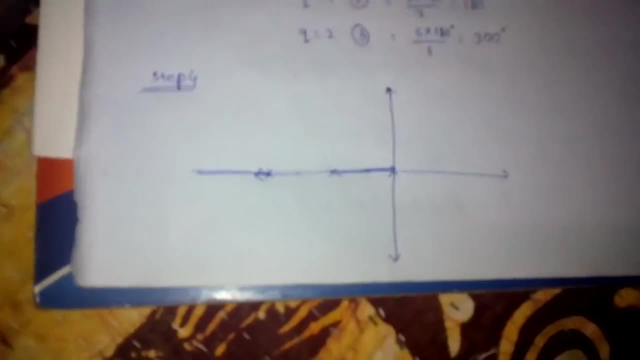 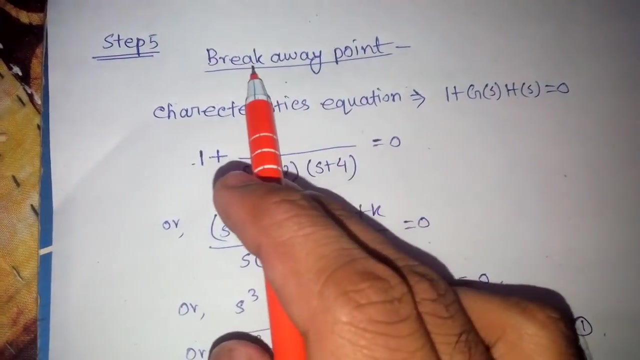 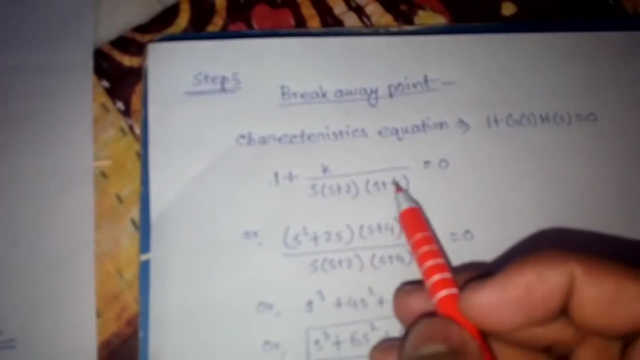 root locus. one is for this and one is for this. okay, so we came to step five, and at step five we have to find out the breaker point. for that we need characteristics equation. that is, one plus gs, hs equals to zero. so one plus gs, hs and gs we are given here and hs is you need to fit with one. 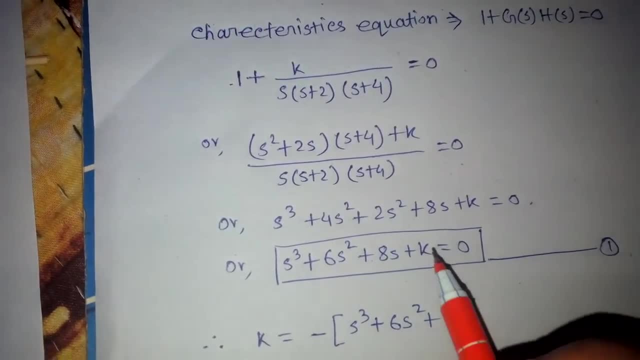 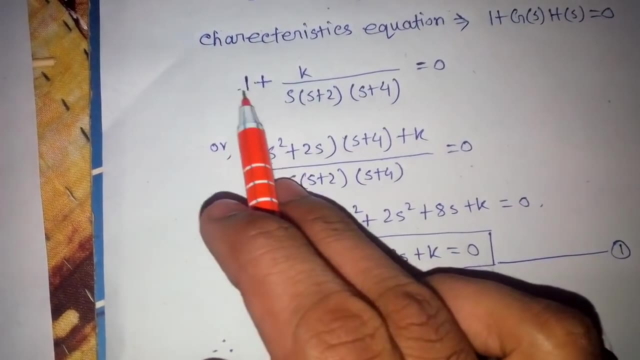 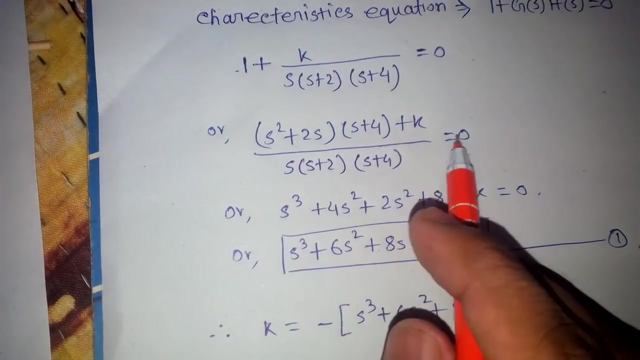 so we just, uh, have a write down the equations, so we just multiply this- this is square plus 2s- into s plus 4. so this i multiplied plus k, divided by this thing, this thing i have written, so this thing will multiply with this and will become zero. so this will be. 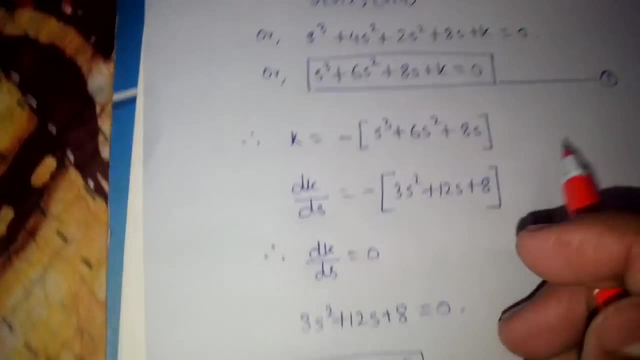 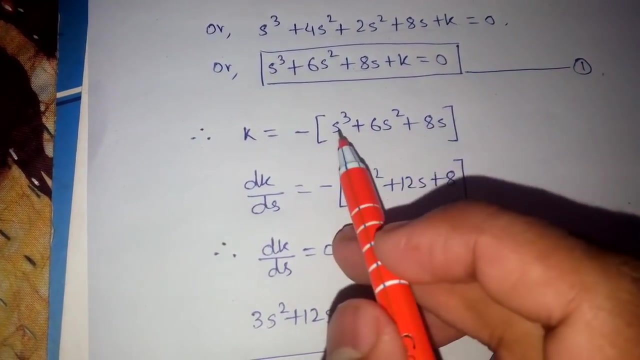 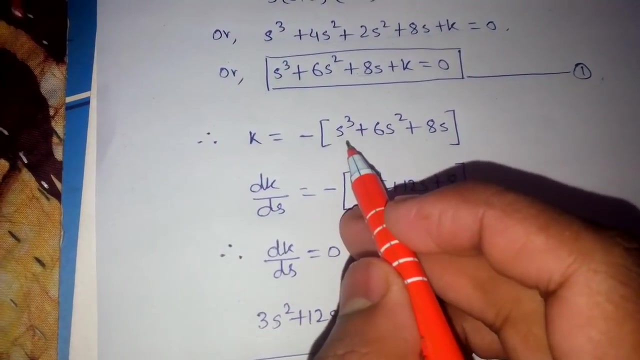 my characteristic equation mean characteristic situation. so from here what we have to do, we have to side k, one side and another the total portion. we will put another side like this. then we will find out the dkds. so after dkds, derivative of this 3s square plus 12s, as you can see, then we have to. 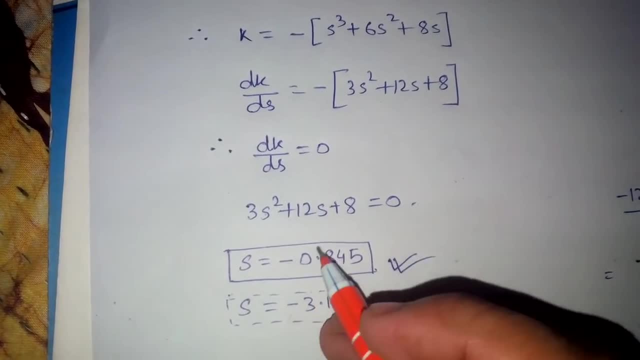 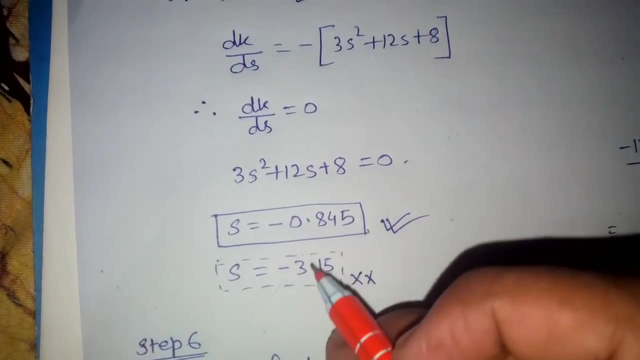 put dkds equals to 0. so when we put dkds equals to 0, from here we can solve the two roots of s. so we can find there. two roots are there. so in between them. so we can see one is minus 0.845 and one is. 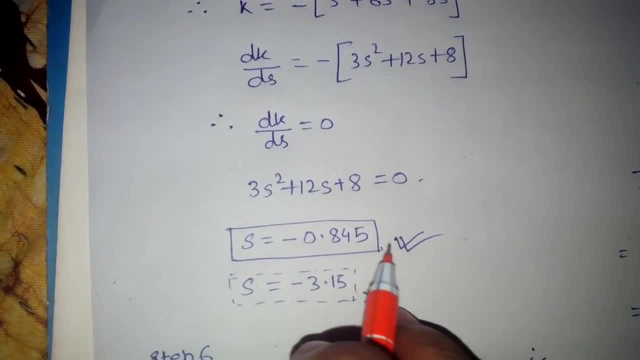 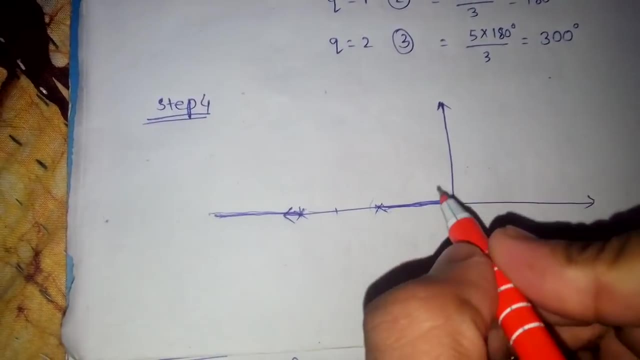 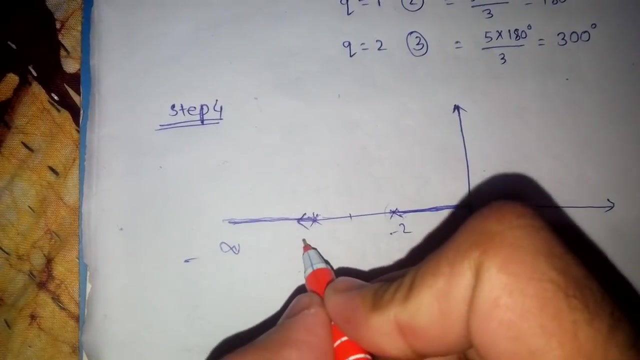 minus 3.15, why we are choosing this as the main root or the main breakaway point. why because in our previous page we have seen that our root locus lies between the 0 and minus 2 and after that infinite 2 minus 4. in between 2 and 4 there is 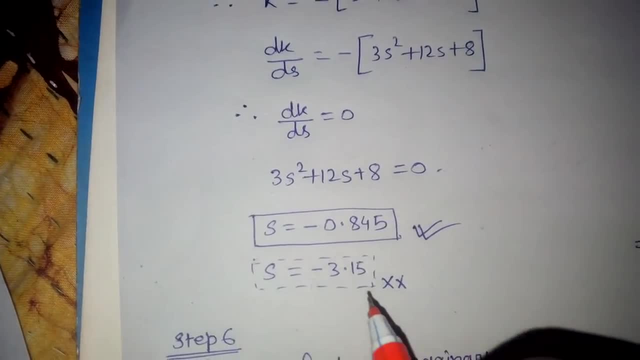 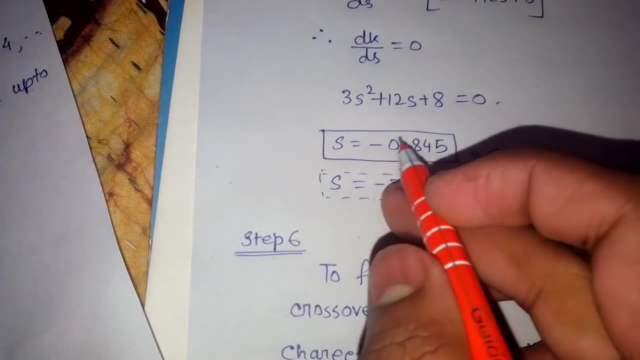 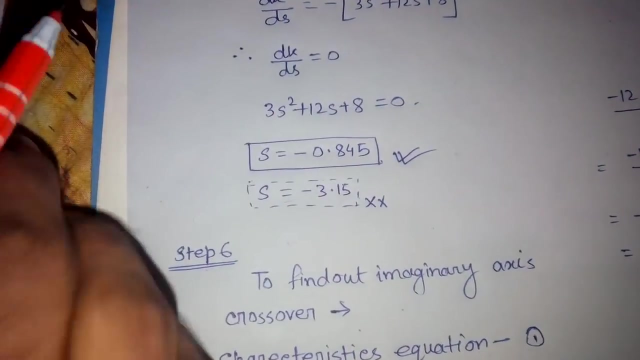 there cannot be any breakaway point. so 3.1515, that is between 2 and 4. so this point cannot be really exist. so this point can be exist because it is in between 0 and 2. okay, so we will move to step 6. to step 6. we have to find out the imaginary axis crossover. 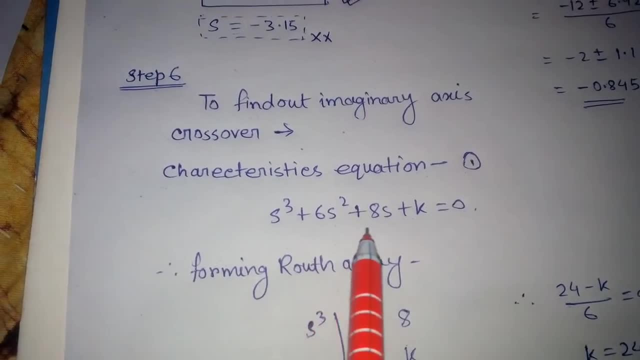 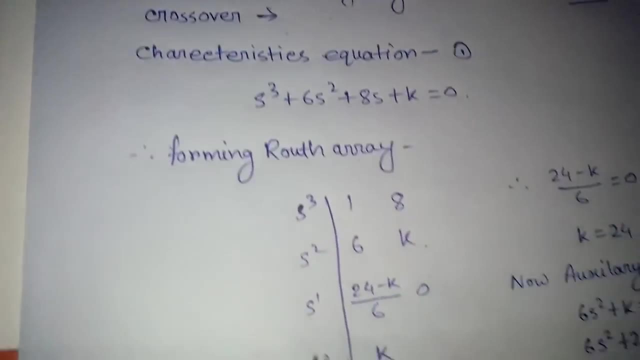 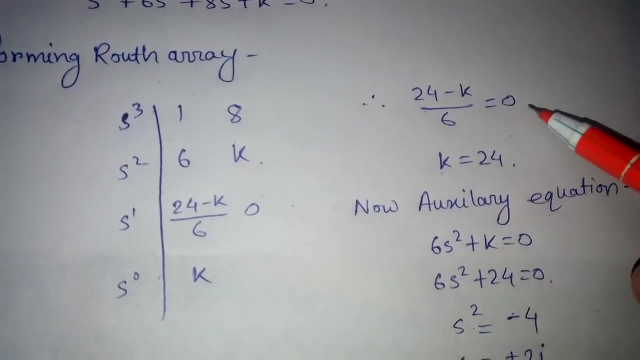 step 6.. so we just write down: the characteristic execution is q plus 6 square. that is, this is q plus 6 square. it is plus k goes to 0. so we have formed the route like this. you can check it. so from here we have make this 0 and from there we get k goes to 24. then we made the. 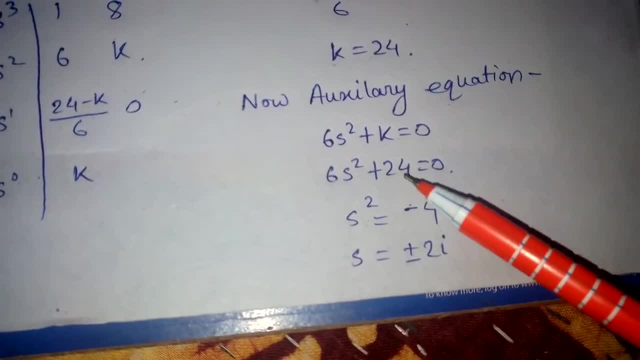 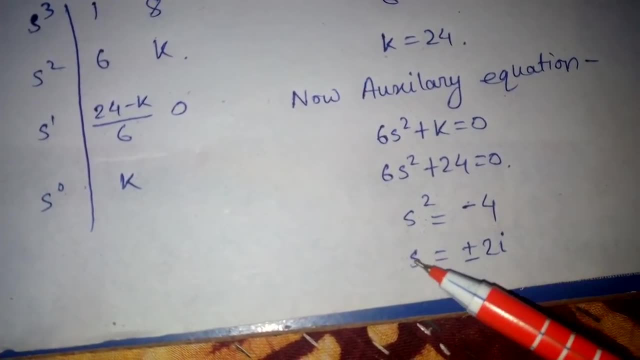 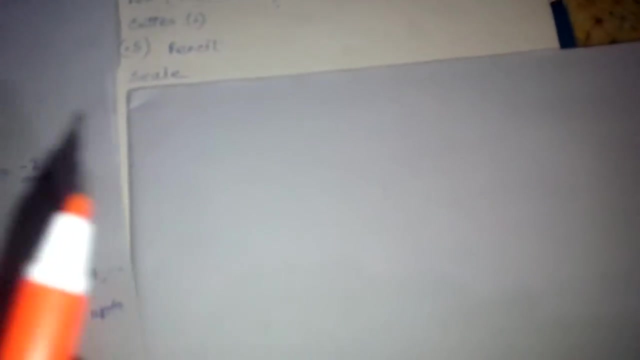 auxiliary equation: 6 square plus k, that is equals to 0, and there we put the value of k 24 and from there we will find out the roots of s. so there is two root plus minus two root plus minus two root plus minus 2i. okay, we'll roughly make uh, step seven, we'll limit. 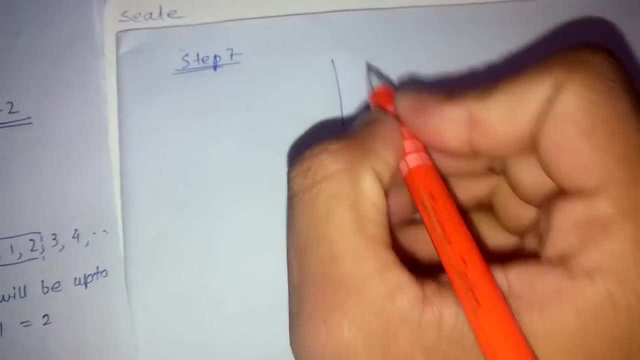 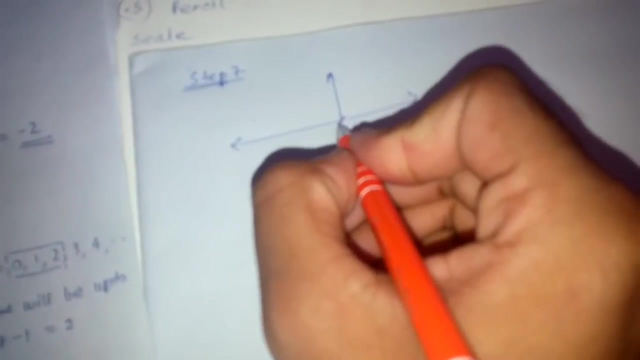 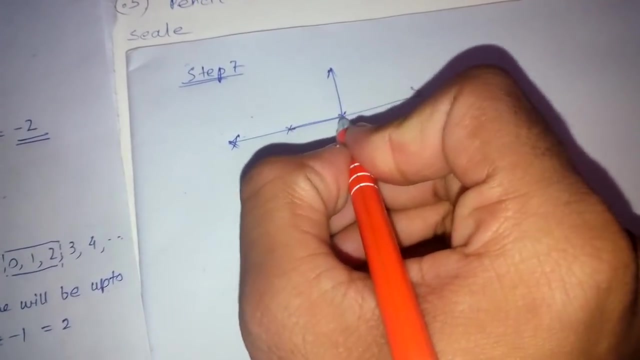 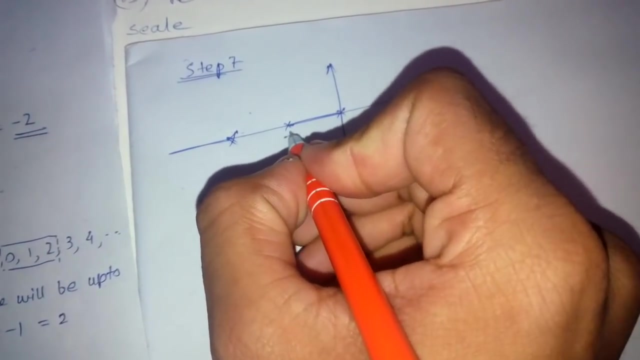 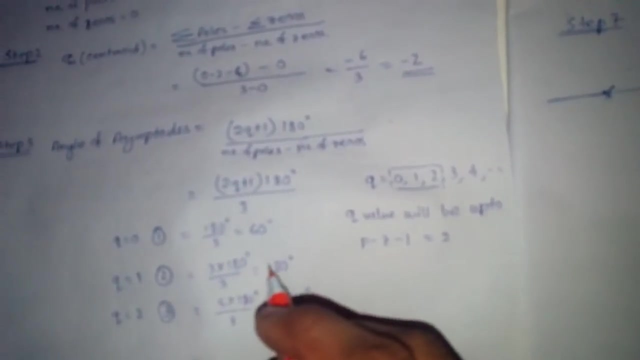 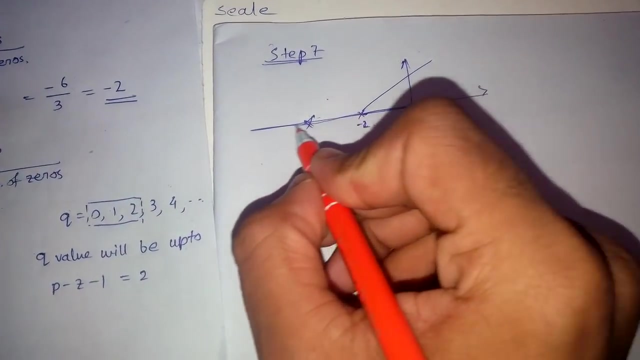 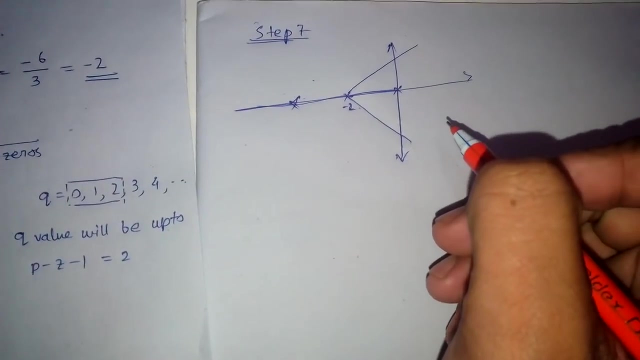 step seven and we'll roughly make a root locus like this. so here is one pole, here just one pole, and here is one pull and there lies the root locus, and there also lies the root locus And our centroid point is minus 2. that means this is our centroid point. So from here we have 3 angular asymptotes that are this: this, this: So 60, 180 and 300 degree are the angular asymptotes. So from here we have drawn 60 degree, This is 180 degree and 180 degree, So this will be 300 degree approximately from here. So, and this is 60.. 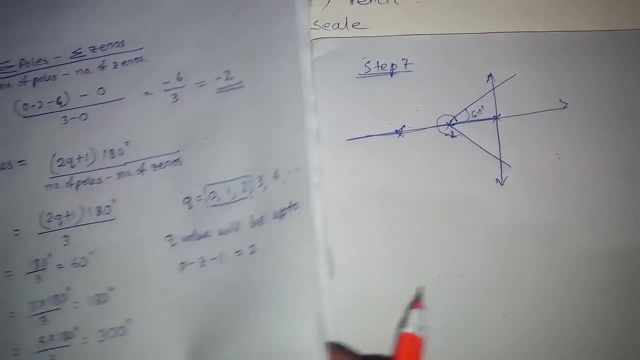 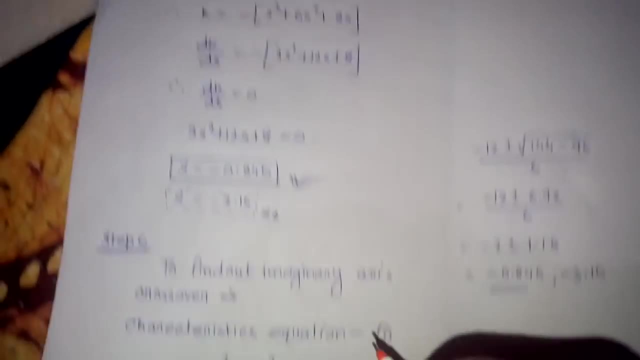 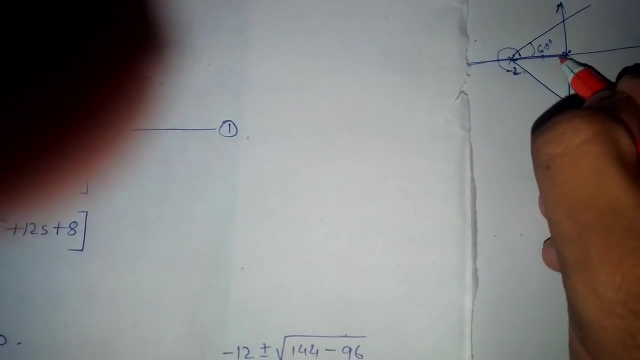 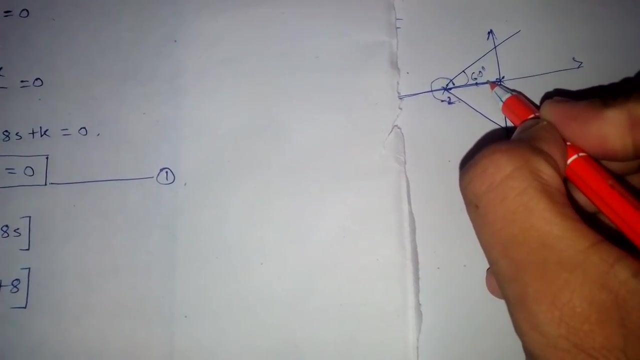 So after that we have completed step 3.. Now we will go for step 5.. From step 5 we have found out the breakaway point. So breakaway point was minus 0.845.. So minus 0.845 approximately. it will be here Here 0.845.. So from here we will just make this and this. 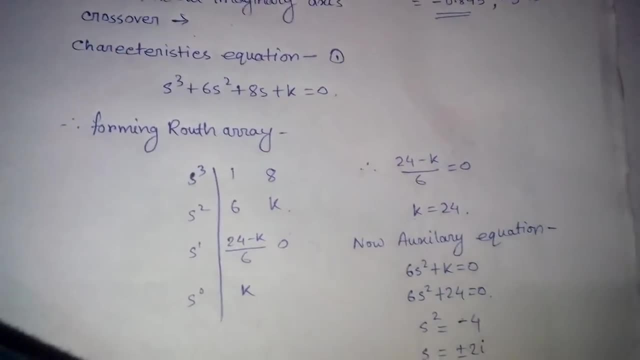 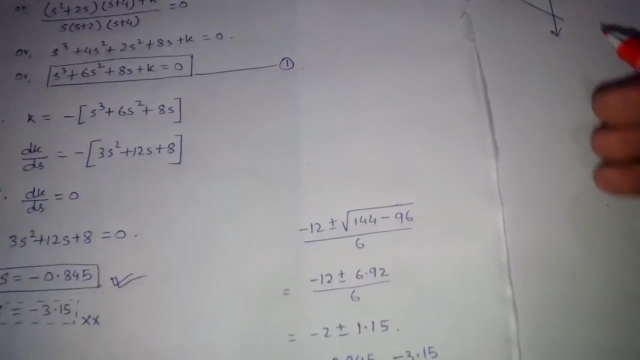 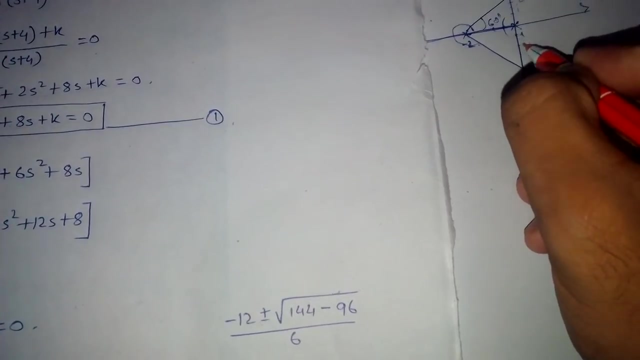 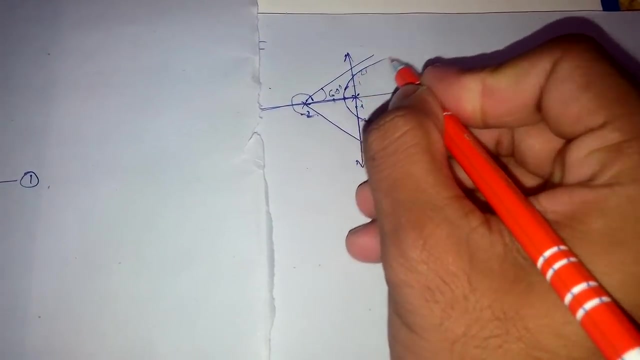 After that we will find out the imaginary crossover That is from step 6, imaginary crossover That will be: is equals to plus minus 2i. So if this is i and this is 2i, This is i and this is 2i- Sorry, this will be minus. So this point will cut through this and that will cut through this and it will go along this angular asymptotes. Okay. 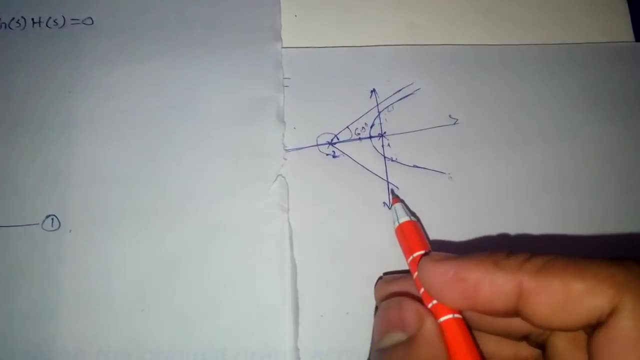 So this is the question And this is the answer, And now we have to put it on just graph you will be given.